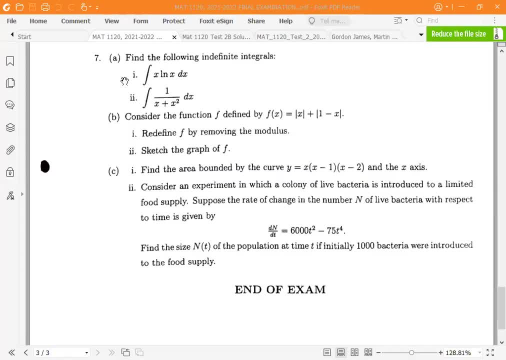 So the question says: find the four indefinite integrals. The word indefinite means there are no limits on the integral, You just integrate and add the constant C. Definite are those integrals where there is maybe two to four. So after you integrate you substitute those. 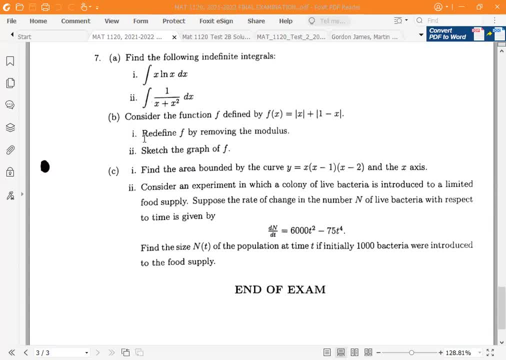 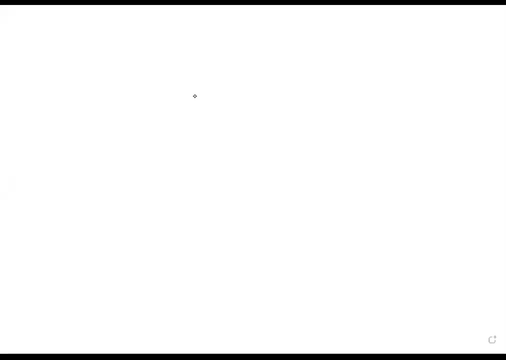 numbers, So you don't have the constant adding. So now we want to integrate X lean X, Okay, Okay. So that's question seven A: integrate X, lean X, BX. So this question, this question, needs to be integrated. Now look, in integration there's no product loop. What is there is? 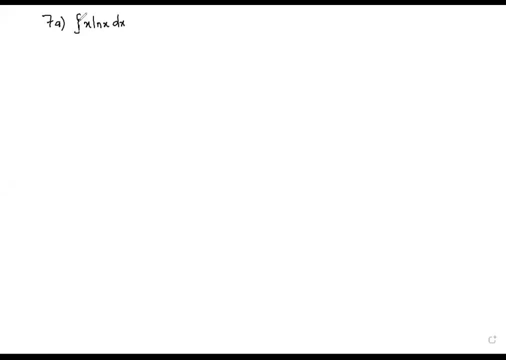 the rule which is called by parts. So we have to integrate this by parts. Okay, What is integration by parts? If you find that you are asked to integrate a product of V and a product of U and BV? If you are told to integrate a product of U and BV, what you do is you separate them. 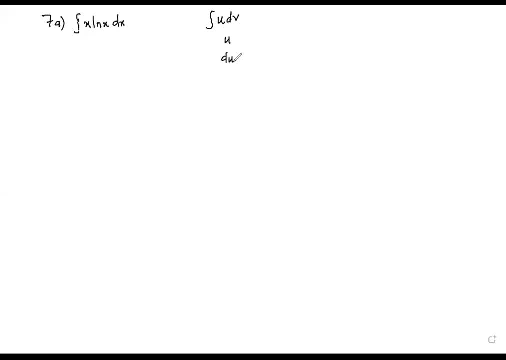 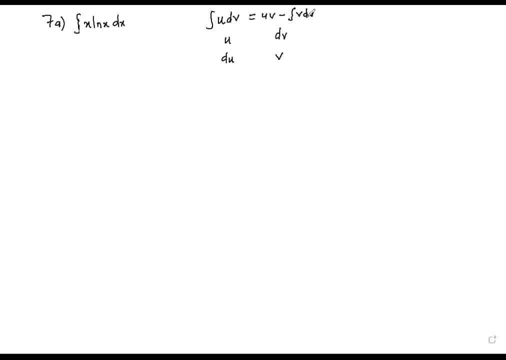 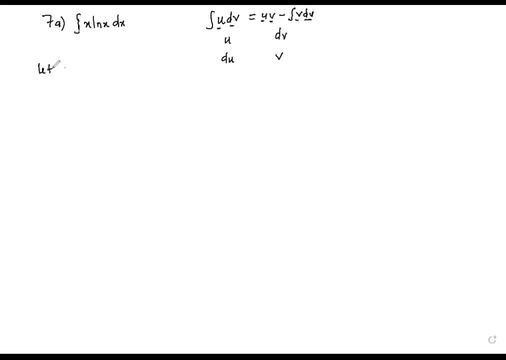 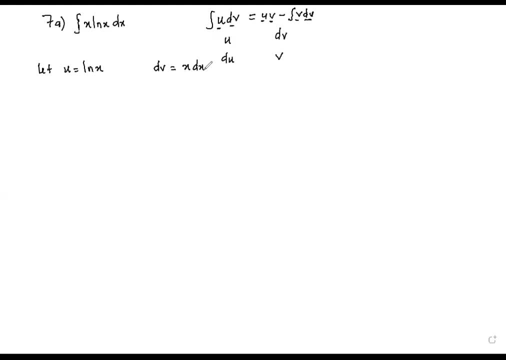 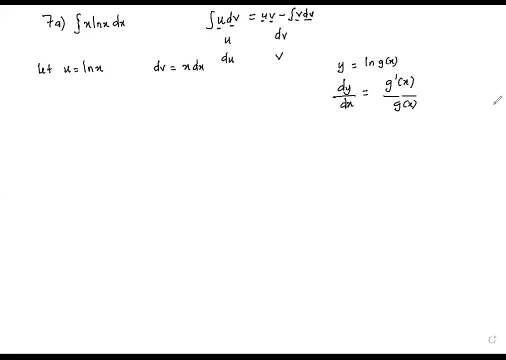 So if we go to our lean x, you see that the g we have is x. So what we'll do to find du dx? to find du dx, we will differentiate x, We'll get 1. And then divide by the x itself. okay, 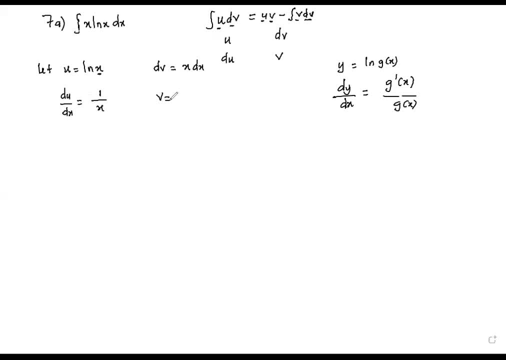 To integrate dv. to integrate dv, you integrate x. So you add The power is 1 there, So it will be 2.. 9. Over 2. So you say: okay, so the integral of x and lean x, dx is equal to uv, which is x squared. 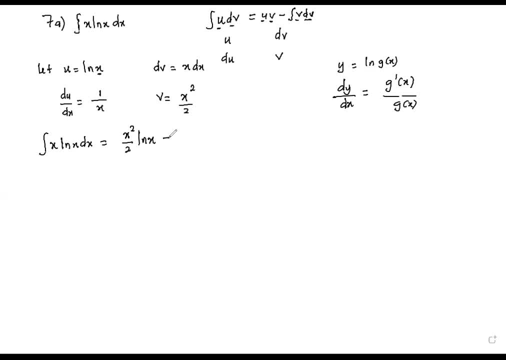 over 2, lean x minus vdu. So that will be the integral of x squared over 2.. And 1 over x dx. Since I'm saying vdu, it means the du must be left with the dx on the other side. 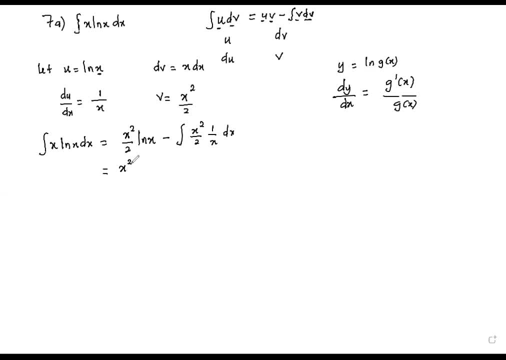 So here you now drop the x squared over 2 lean of x minus the integral of x over 2 dx. Okay, Okay, Okay. Then from there you have x squared over 2 lean of x minus. You integrate x again. 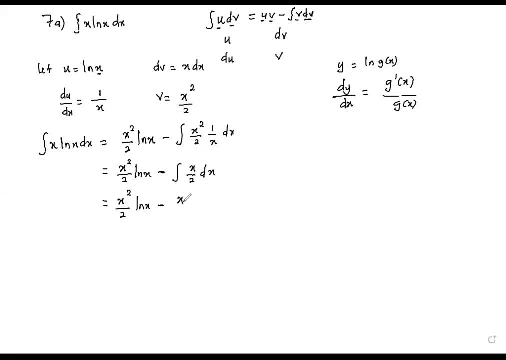 It will be x squared, Then the square will multiply by the 2 to make it 4. And then plus C, So that will be the solution. So this should be the easiest method, because it's like product 2. Except it does not differentiate the du right. 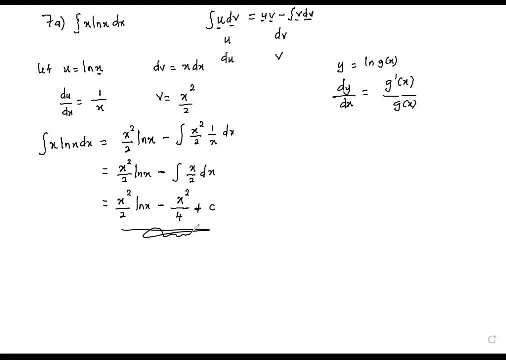 Right, except they're not differentiating everything. we just differentiate one and integrate the other. you see, hello, i don't understand where the x squared is coming from. yes, this x squared over two and the other x squared over. i don't understand where the squared things are coming from. so we are. 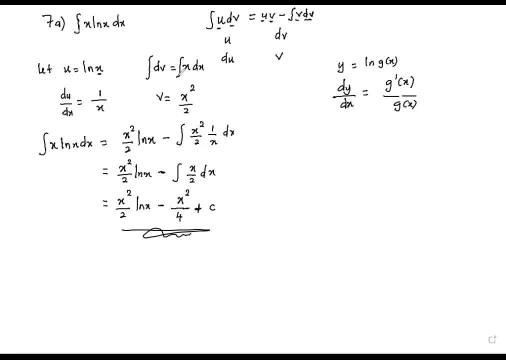 integrating dv. oh, i still don't understand. let me wait for my examples. okay, wait, do not integrate this. you integrate this. you add a one to n and divide by n. that's not the point. thank you, i think i don't understand. sorry, i have a question. 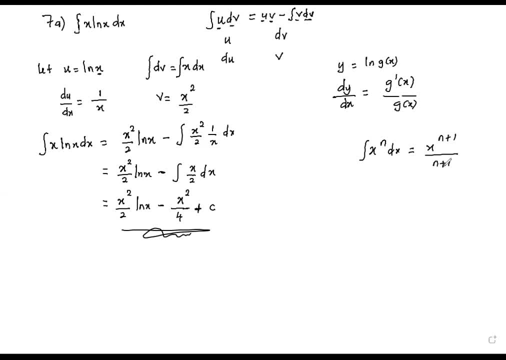 why didn't we integrate? why did you use uh use substitution here? because it can't be used here. so user fusion requires that when you differentiate the u, so u. substitution requires that when you differentiate the u, u because you can't be used here, so u. substitution requires that when you differentiate the u. 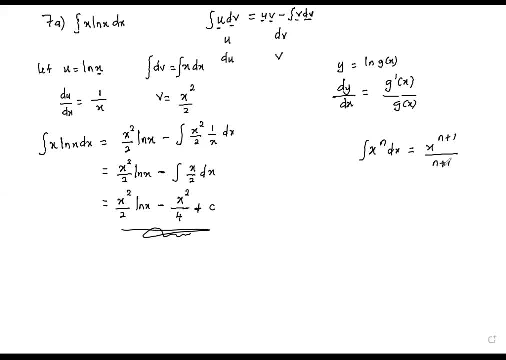 the deal you get is also there in the function. But when you differentiate lean, you are getting one over x, but what we have is x there. So it's kind of tricky. Okay, maybe when we find some more we'll begin to like it. 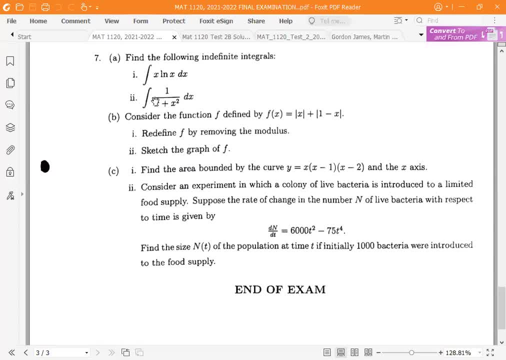 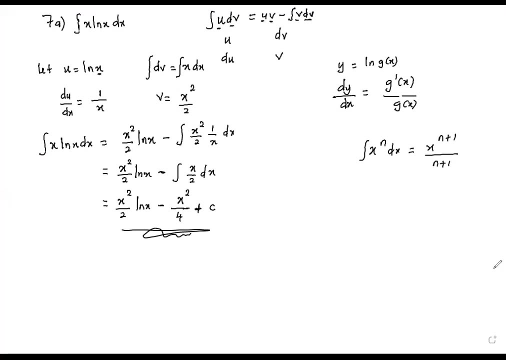 Let's go back. Here's another one: The integral of one over x plus x squared dx. The integral of one over x plus x squared dx, Part two: The integral of one over x plus x squared dx, Here by parts, cannot work. 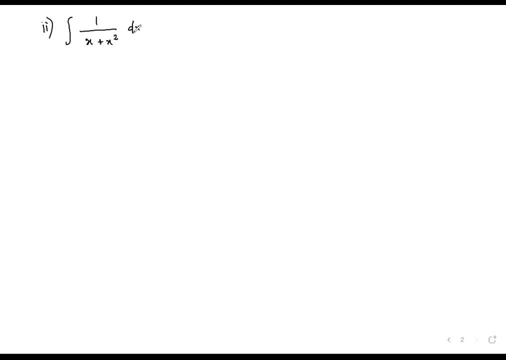 U substitution cannot work Because the derivative of the denominator is not anywhere near the numerator. In fact we can't see it here. So what we do is we will resort to using partial fractions. So we'll write this integral as the integral of one over x squared dx. 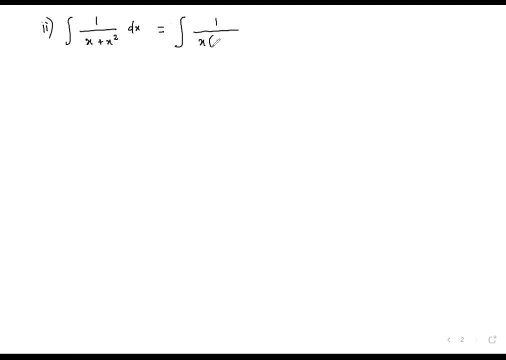 So we will write this integral of one over x squared dx. So we'll write this integral of one over x squared dx, The integral of one over x squared dx. So we'll write this integral of one over x squared dx over x. 1 plus x will be x. 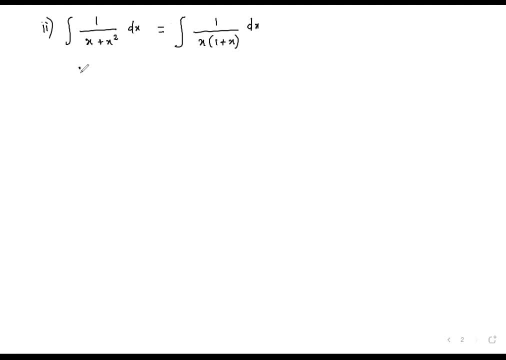 And then let's pick now the 1 over x, 1 plus x. We pick it and break it into partial, So it will be a over x plus b over 1 plus x, So the partial that you can be asked in these courses. 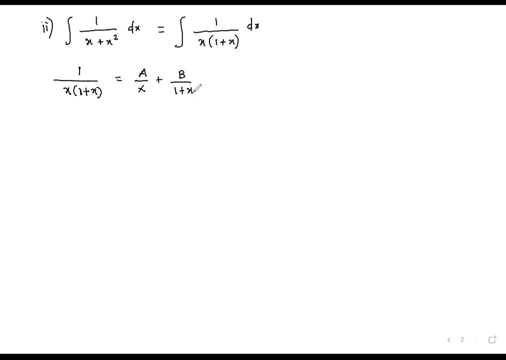 that we are doing is a linear kind of partial, where when you separate them the product has x's with power 1's. So I just separate the first one under a, the second one under b, if they were 4, under c, under d. 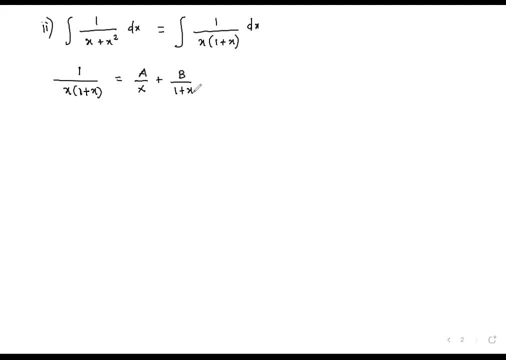 So the target is we are solving for a and b. So to do that, you multiply and throw out by the common denominator, Which, Which is x, 1 minus x. OK, So when you multiply you see that this one and that one. 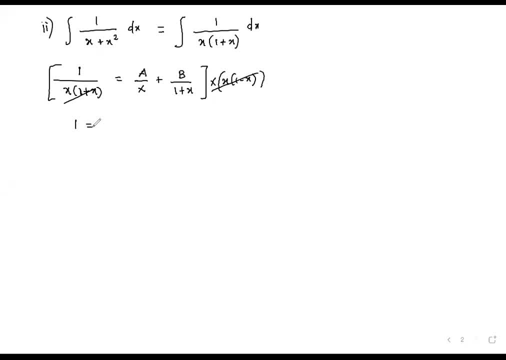 will cancel, So we'll have 1 on the left. Sorry, why are we multiplying by 1 minus x but not by 1 plus x? Oh, it's 1 plus x. Thank you for that. Then for the a. 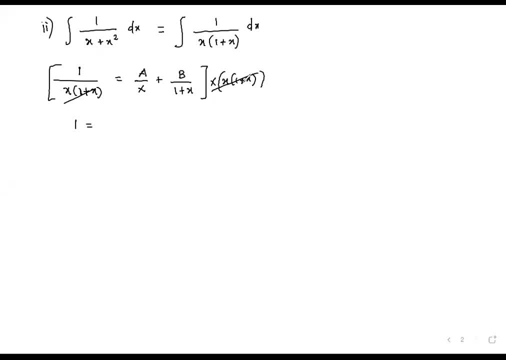 So the a part, the a, will only come and cancel the x. So it means that the 1 plus x will remain, And on the b the x will remain. So this is the equation that we remain with. So at this point we now expand further. 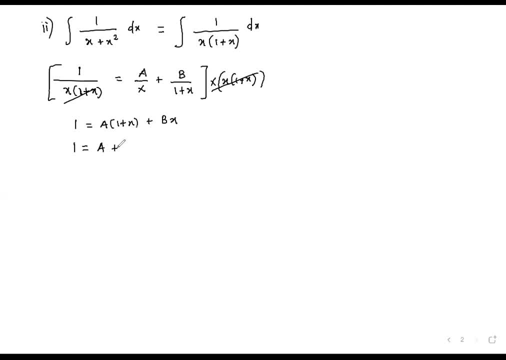 So we'll have: 1 is equal to a plus ax plus bx. OK, OK, OK, OK, OK, OK, OK. When you reach here now the coefficients of x, to respect the path, you equate them If on the left I pick a constant. 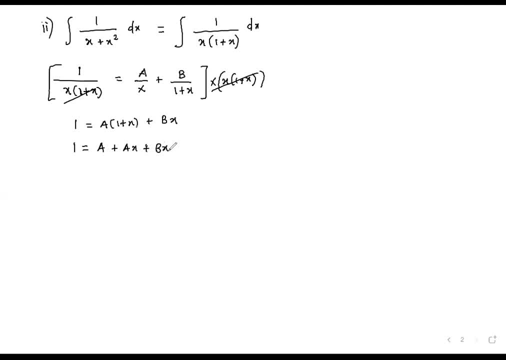 On the right, I should go and pick the constant. A constant is that number that was being multiplied by x. If, on the right, I pick a number being multiplied by x, I should collect all such numbers, put them together and equate them to a number being multiplied by x. on the left: 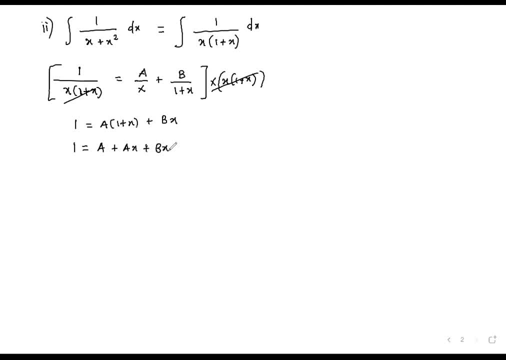 Now, in our case here, the number on the left is 1, not being multiplied by x, And on the right is a not being multiplied by x, So it means that a is actually 1.. And then ax plus bx should be equated to 0x. 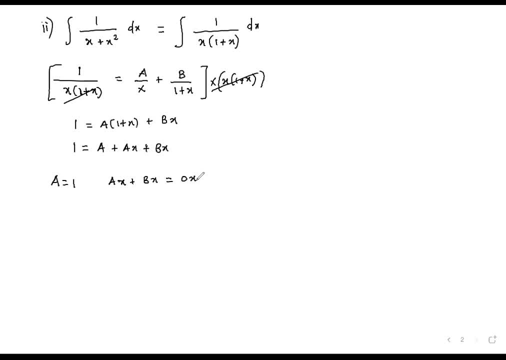 Because there's no x on the left. it means that the equivalent of x on the left is 0. So when this happens, it means that a plus b should actually add up to 0, because they are the coefficients of the x that we are using on the left. 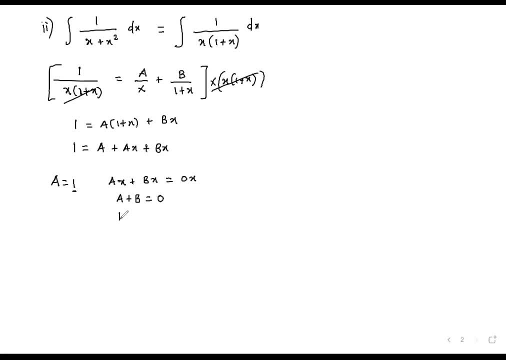 But we have said, a is equal to 1.. So if we substitute 1 here plus b, it must give us 0. That happens if, and only if, b is equal to negative 1.. So now we get back and say: okay, so what do we have in the integral? 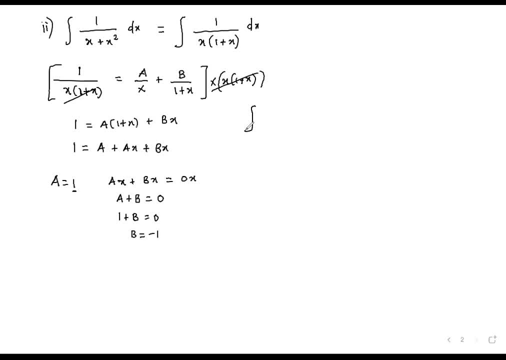 Wait, sir. How is a equal? It's equal to 1. again, I didn't get that. So if you are saying this is equal to this on the left, then a should be equal to 1, because that's the only constant we have on the right. 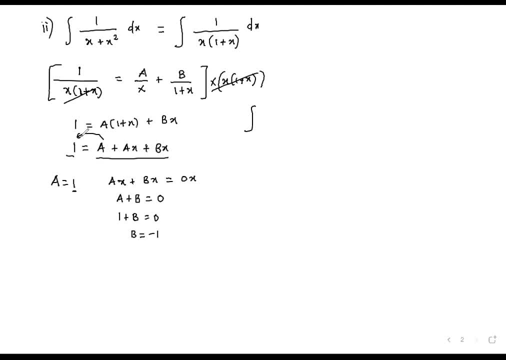 The other ones on the left should be multiplied by x, And yet we can't see anything here being multiplied by x on the left. I don't know if it makes sense. Yes, it does, Oh good. So when we go back, what was the product? 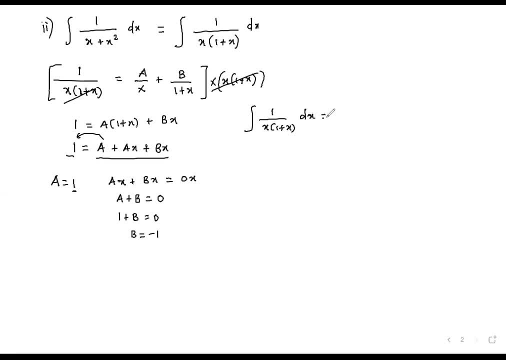 It's now no longer a product. So we have the integral. So we have the integral, So we have the integral Of 1 over x plus b, which is negative, 1 over 1 plus x, bx At this point now, that is when we use u-substitution, okay. 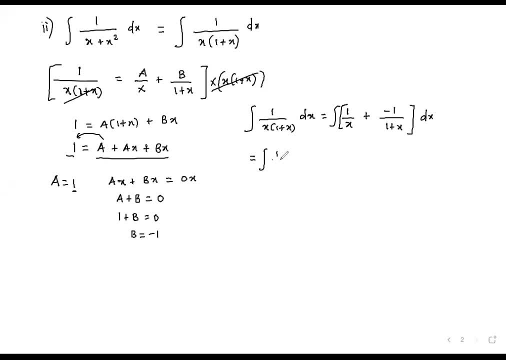 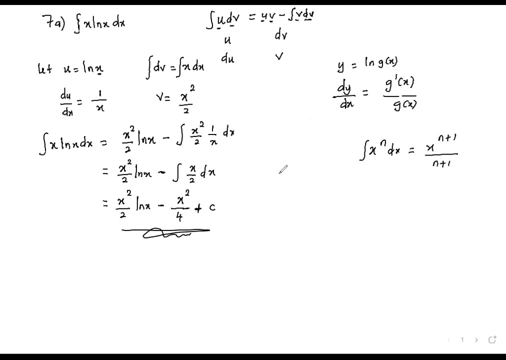 Because now the integral can be separated. It will be 1 over x bx, minus 1 over 1 plus x bx, Like that. So meaning for the first part, you know in the previous part the derivative of lin x. 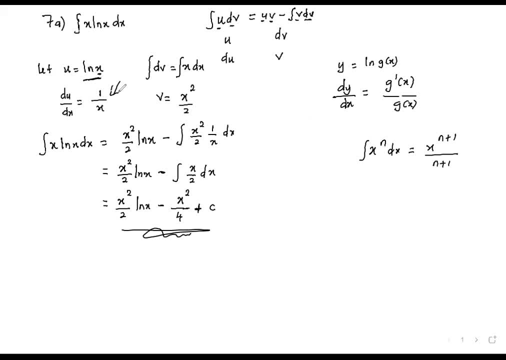 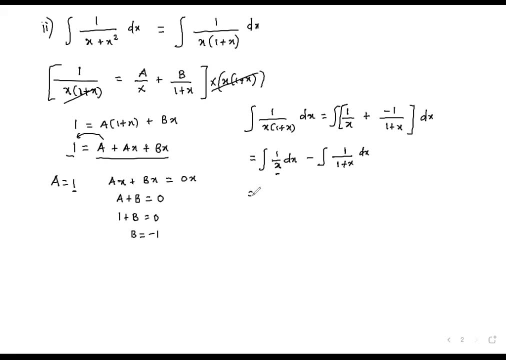 Was actually 1 over x, So that if we integrate 1 over x, you'll get lin x. So the integral of 1 over x is actually lin x Minus. the integral of 1 over 1 plus x is also lin 1 plus x. 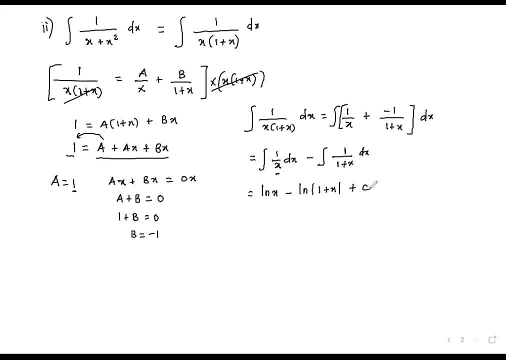 And then plus c. So I'm putting the absolute, Because the integral emphasizes that lin must be defined And lin of a negative number Is undefined. So we are restricting a negative. We don't want to use a negative here, And so we restrict it. 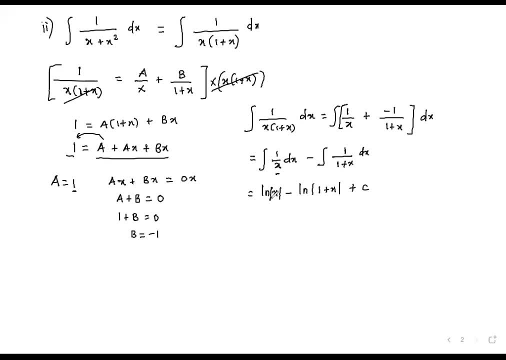 So I have a question. Yes, What's the question? So what method is this, The one that you've used here for this? Like the partial Fraction Differentiation, Like what's the code? It's called partial fraction integration. 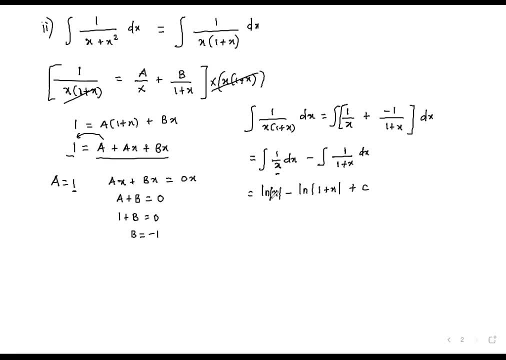 Okay, Thank you, sir. So that's how you call the, The integral. So the method itself is actually by parts. I think I think you guys have done the by parts and there are so many questions that I guess. so I think in all the tools you should have that in the main direction. 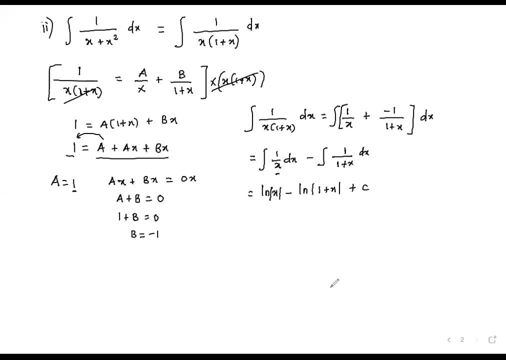 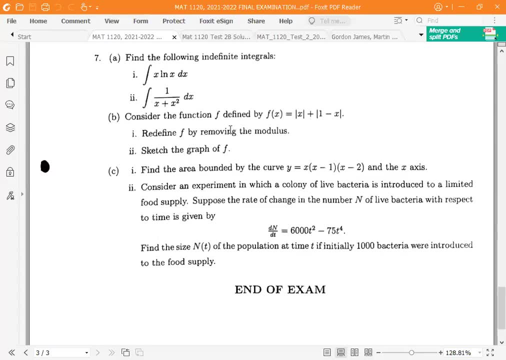 I know you enjoy it. I think Go on. So that's what's next. Next we have considered a function, M Defined by F of X is equal to the absolute value of X plus the absolute of one minus X. Then part one says: redefine F by removing the word. 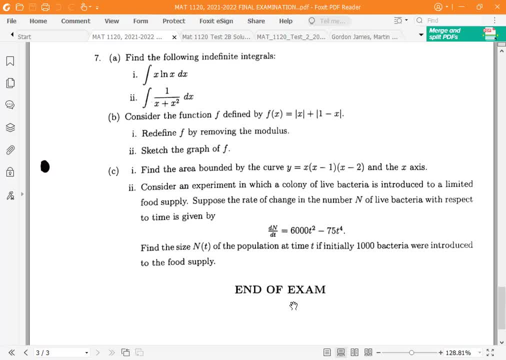 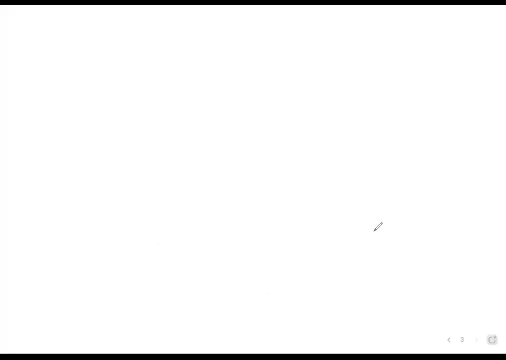 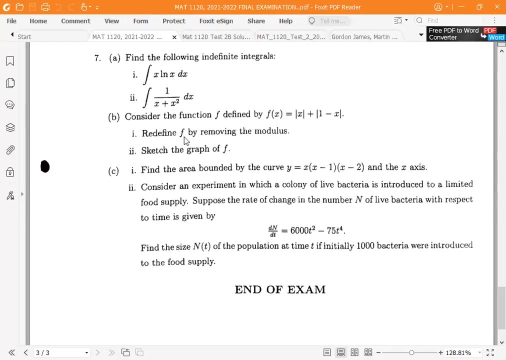 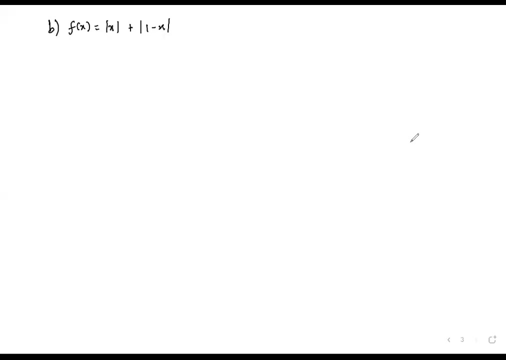 And then it's good to go. So absolute of X Plus after the one minus X. No, So B? F of X is equal to Absolute of X plus absolute one minus X. So let's pay attention, I think, on this. person has trouble with people for some time now, including. 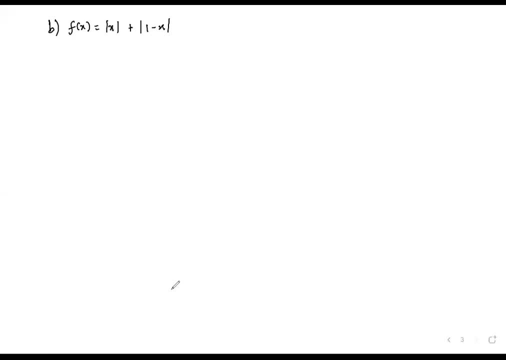 Including: I feel like you must, Very, they must. I feel like you must, Yeah, In grouping that, All right. So How do we define this? You pick the best part, The absolute of X. By definition, it should be: 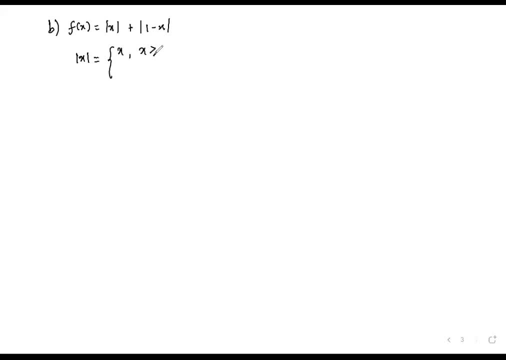 X If X is greater or equal to zero. I don't need simple there, Or it would minus X If X is less than zero. One thing to note is that The greater or less part does not go with the negative. The negative sticks on the. 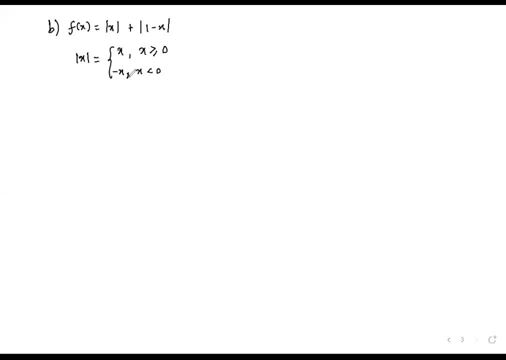 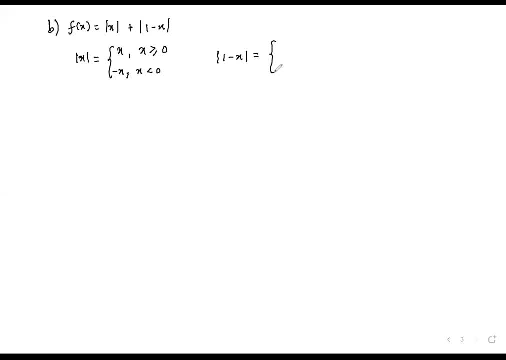 So when you say Absolute of one minus X, It will be one minus X, Such that one Minus X is greater or equal to zero. It will be minus One minus X, Such that one minus X is less than zero. 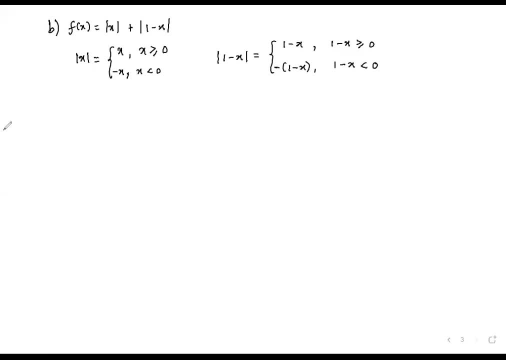 This is the point that I was saying: That When you get To the, To the inequality here, There's no negative. This is one minus X The way it was inside. This is one minus X The way it was inside. 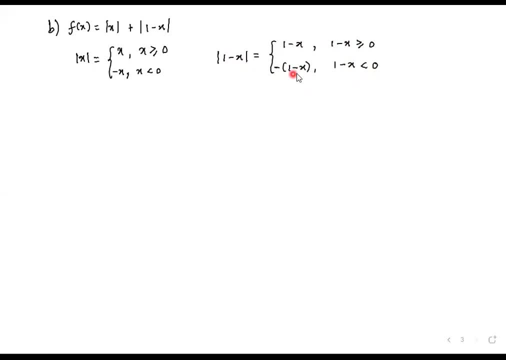 The minus only affects this part And not The incorrect part. That's the point that I was saying. Then now we come back, and So This Will be One Minus X. If I have a Small question, 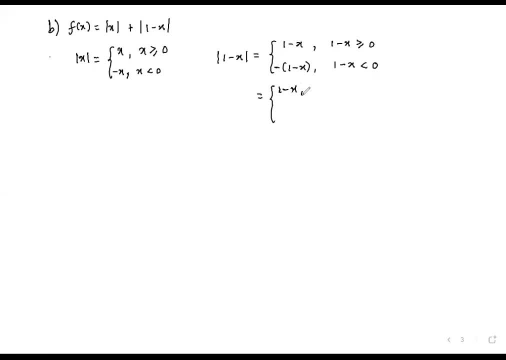 Can I ask? Yeah, Okay, So Usually when Defining questions, They Sometimes they Put a plus And sometimes they put a minus. Does that Mean anything, According to How you're Solving? Yeah? 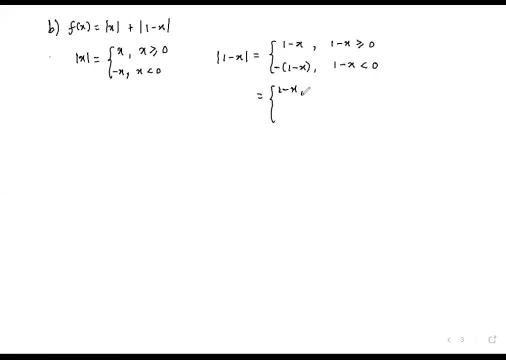 It will mean a lot. So you see Where it Matters, How it will be. Yeah, Yeah, Yeah, Yeah, The Well, Okay, So here We have Minus X, Greater or Equal to minus 1.. 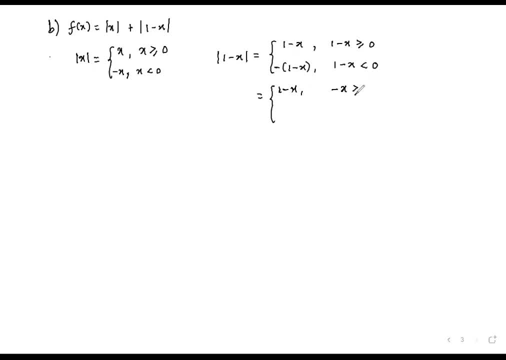 We Can Expand, So we have minus 1.. Last, X Minus X, Less than minus One, Which can be simplified. Further One Minus X If X Is less Or equal to one. 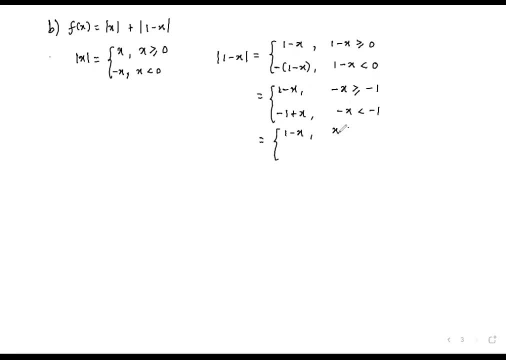 X Minus X Is One Plus, and to x minus one if x is greater than one. so i'm just dividing on the inequality here by negative, by negative whenever it is changing. you know, whenever i divide by negative on the invite will change the direction. 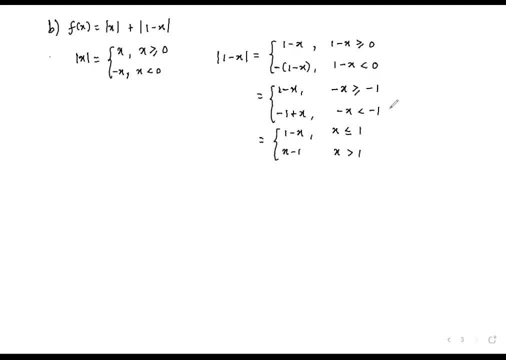 so from there we now go back to f, say okay, so our f of x redefined is going to be of this kind, the first thing we'll do: between the numbers we have, we have zero and one, so one is bigger than zero, so we start with zero. so we say when x is less than zero, 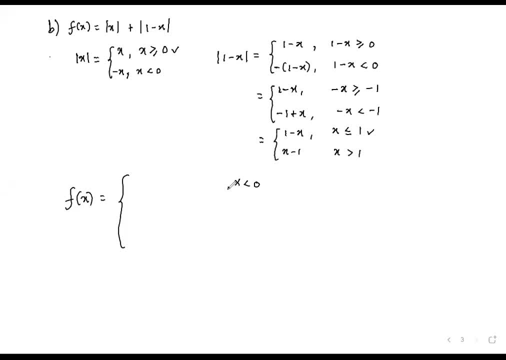 what is the situation? the first part, when x is less than zero, the first part is saying it is going to be negative, negative x, then we get that plus. so we put a plus there. when we put the plus there, we come where else where x is less than one, because zero x is less. 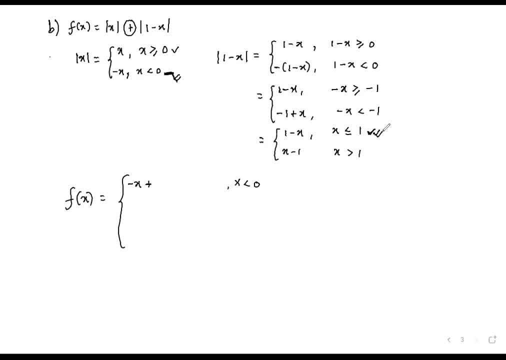 than zero. so if x is less than one, it's possible that that x is less than zero of the one. so whichever x is is less than zero, automatically it's less than one. so from this part you pick the top one, which is one minus x. then there's another interval where you are less than one but above zero. 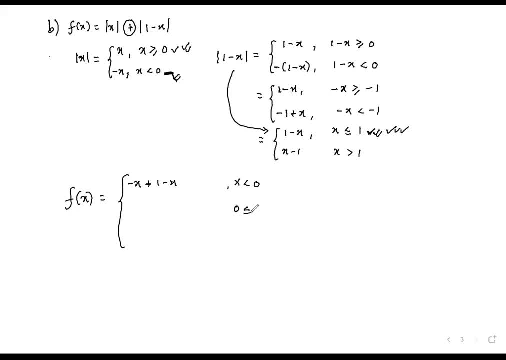 okay, so say, zero is less or equal to x, but less than one. so i've picked this part. but we know that there are some numbers bigger than zero but less than one. so when x is bigger than zero, this function here is x and this function there is still less. 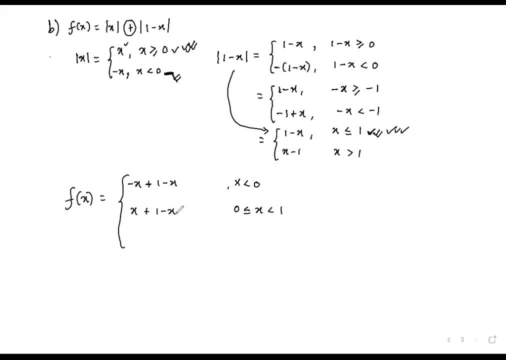 than one, then when x is bigger than one, greater or equal to one, from this part you pick the one that is bigger than zero, because if anything is bigger than one, automatically it's bigger than zero. so we have x plus x greater than one. so here we'll pick this one. 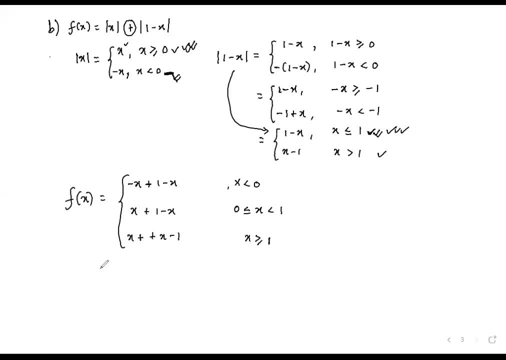 which is x minus one. so what's meaning now is just to simplify. so it will be one minus two x if x is less than zero, and x minus x is zero. so we just make one if zero is less than equal to x, less than one, and then we'll have one meaning. we'll have two x minus one if x is greater, equal to one. 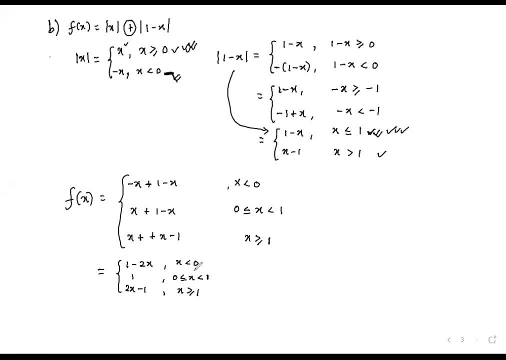 like that. so even a different method is the simple. this is really that's for this, so that's how it's counted And from here now it's a piecewise function. So you can even escape: It's a piecewise function. It's been easy, Remember. we take that and we say we have. 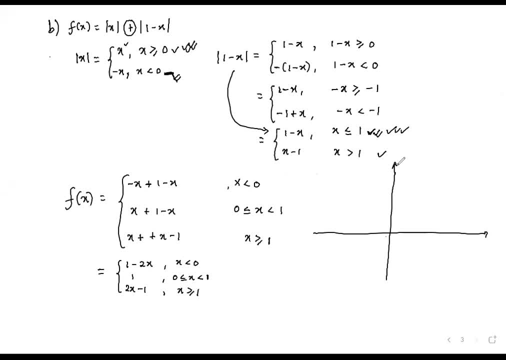 done piecewise function. So here's where we are now. So we have 0.. We have 1.. So between 0 and 1, y is 1.. So you draw a straight line here. You want not to include it? 0 included, OK, This interval Then when x is less than 0,. 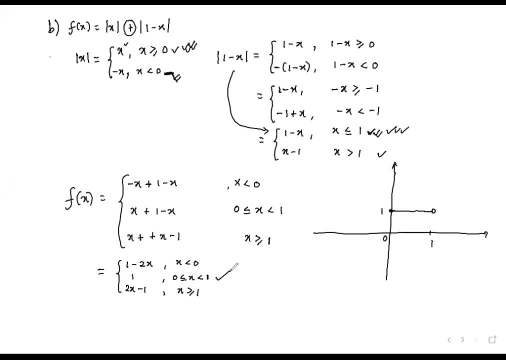 you have 1 minus 2x. So meaning goes like that. It goes like that. And then when x is greater or equal to 1, we have 0.. plus two, X minus one. close, That's a graph. So I have a question. 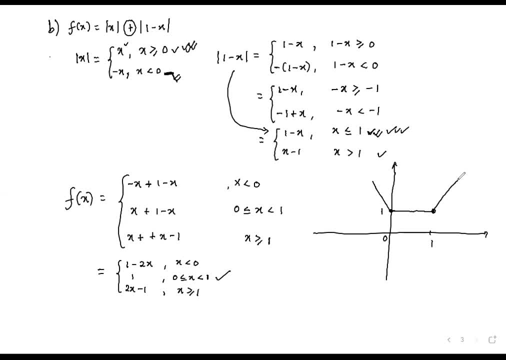 Yes, How did you know the direction where it was going? if it's going up or down, So one. there are two indicators. The first one is that if the gradient is negative, if the coefficient of X is negative, then it's going down this way. 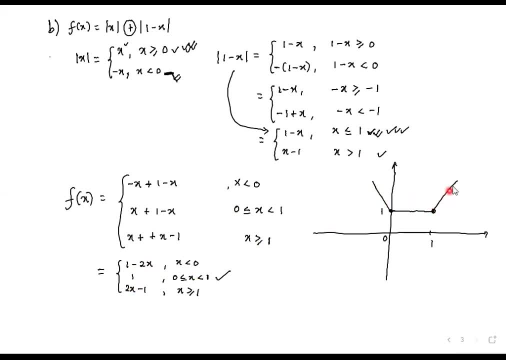 If the coefficient of X is positive, then it's going up that way. Well, if I don't know anything about that, then I take a number less than zero. Say you pick negative one and substitute in this function, So you will have one minus two minus one. 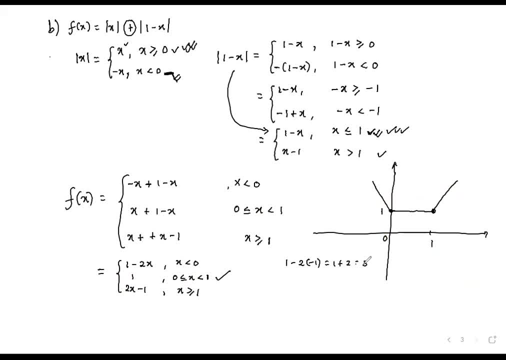 which is one, Two plus two, you can go to three. So three is above one. So it will tell you that they're going up. If you pick positive two, the other side again, you get a number bigger than one. Then you know the direction. 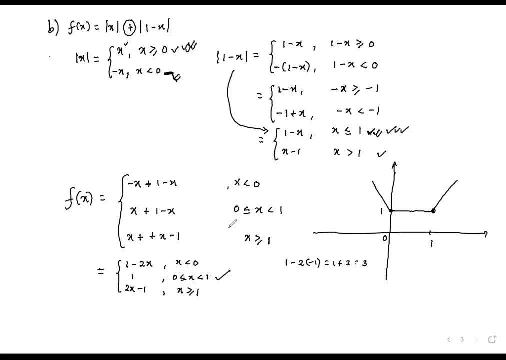 Meaning. you can also use the way I've said about the. let me say negative two X, because it's negative, meaning it's going down, And then positive two X, it's going up, And then one is a flat line. Yes, 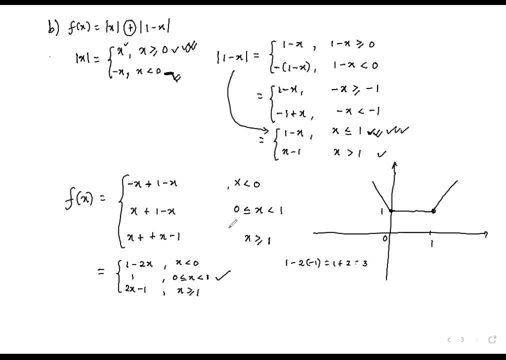 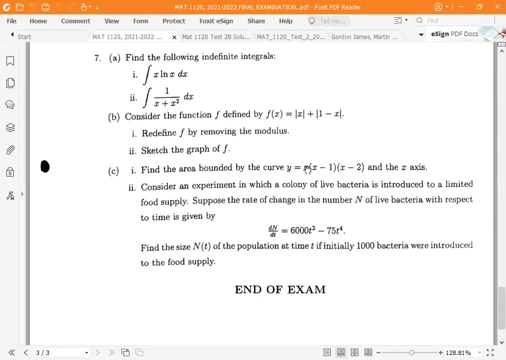 Oh, thank you. Then find: the area bounded by the curve Y is equal to X, X minus one, X minus two and the X axis: X, X minus one, X minus two and the X axis. So if you look at this function, X, X minus one, X minus two. 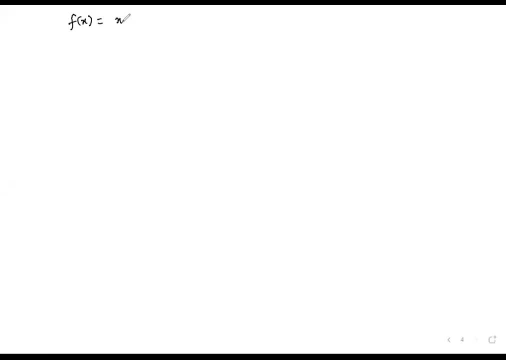 F of X is equal to X, X minus one, X minus two. This is a polynomial that's already factorized. So we go straight to the sketch. We find the Y intercept by putting zero wherever there's X, So we'll have zero. 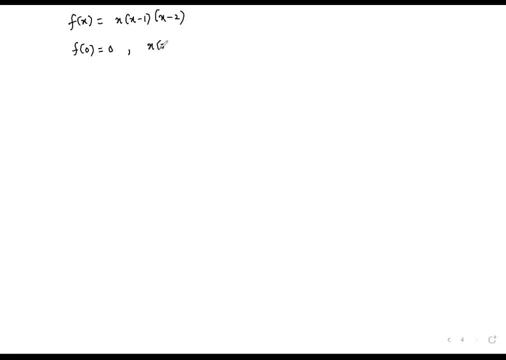 And then we equate the whole thing with zero. We find the X intercept, So we'll have X, zero one, X one and X two. Then we start to find the Y intercept, So we'll have X, zero, one, X one and X two. 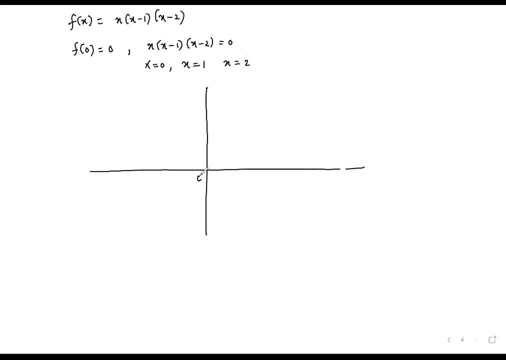 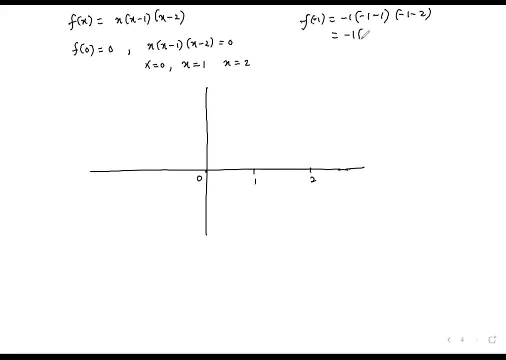 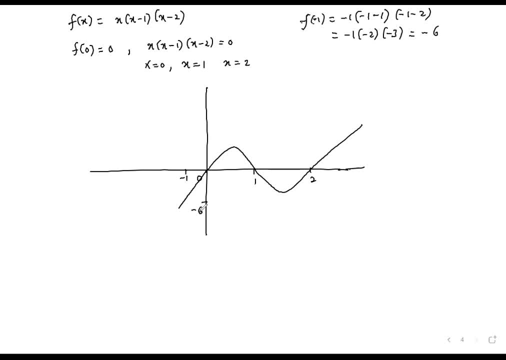 So now, from here we can go back and expand the function. So for the sake of integration, we expand it. So it will be X and then X squared minus two, X minus X plus two, and then this will be X three minus three, X squared plus two, X like that. 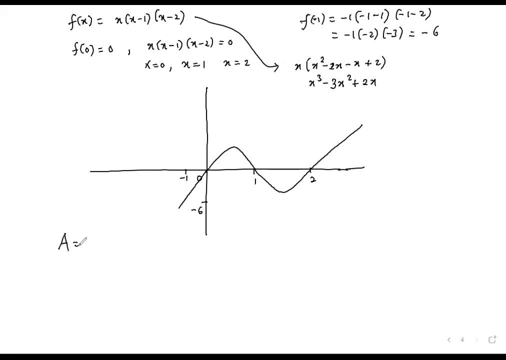 Then now you say the area is going to be the integral, Let me change the ink. It's going to be the integral from zero to one, From zero to one, of this curve minus this line. so the curve is x3 minus 3x, squared plus 2x, and then minus this. 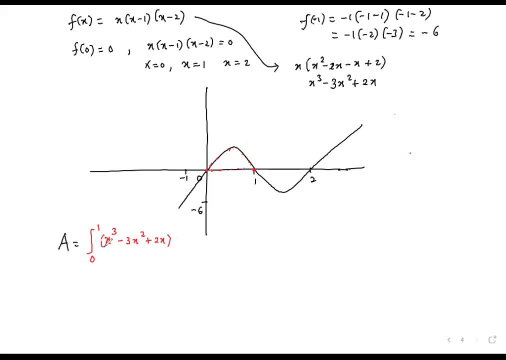 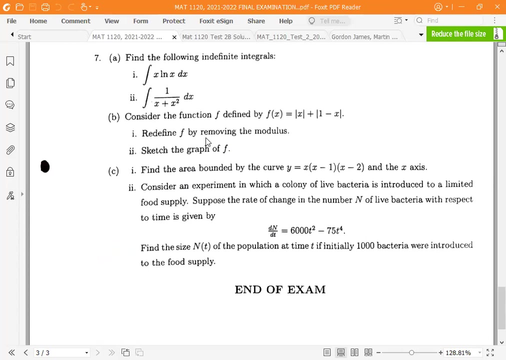 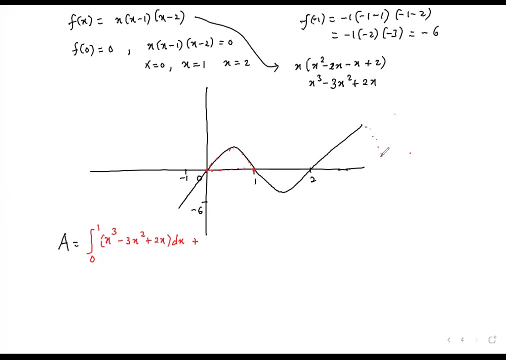 line is zero, so we don't do anything there. but the x plus the function says: uh, you should find the, uh, the area, you should find the area bounded by this curve and the x-axis. so it means that we are done actually, because this other piece is not bounded. there is nothing coming down here, it's just open. so the only area i want to find, 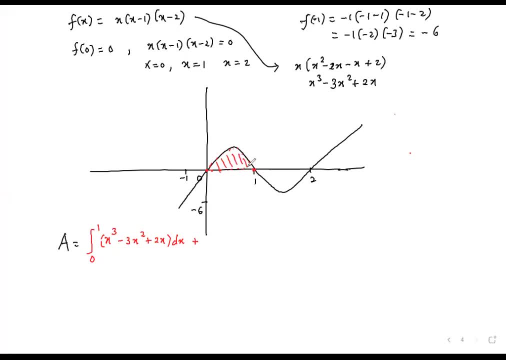 is the area of this region which is what we have here. so just say: equal to. we now integrate, it will be x4. to integrate, you add the one to the power and divide by the number. you get minus 3x3 divided by 3, plus 2x2 divided by 2, and then integrate from. 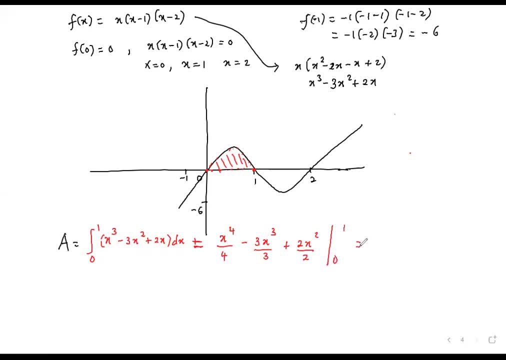 0 to 1. so i'm going to substitute 1: 0. so this means that we're going to have x4. work out a bit: x4 over 4 minus 3 over 3, they will cancel. so we'll have x3 there and then 2- 2. they'll cancel. 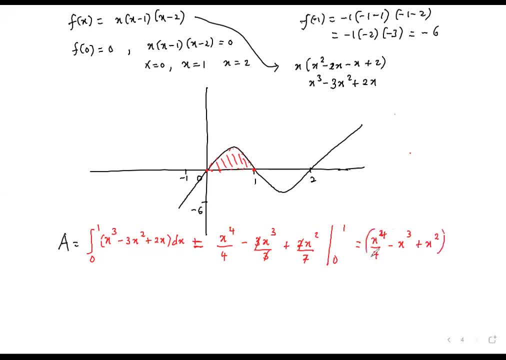 so we'll have x squared here, and then this: we substitute 0, 1. so we start by substituting 1 throughout wherever there's x. so we'll have 1 over 4 minus 1 plus 1, and then minus, you substitute 0. 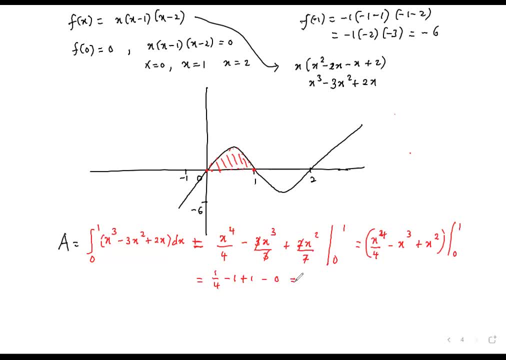 throughout. so we'll have 0. so this means we are getting 1 over 4 units squared as an area. remember, area will support the unit square, so to sketch a polynomial, it's a skew that we all have. the only thing that we lack is factorization. now, this one came factorized, so no execute. you can easily find the. 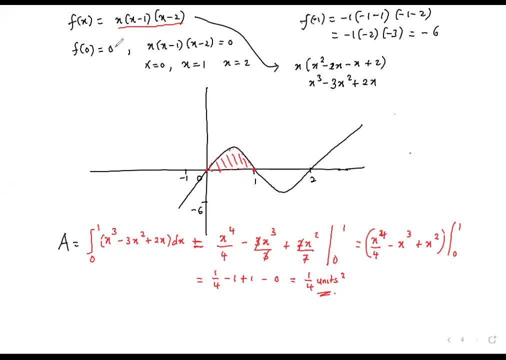 x-intercept but just equating to zero, you can find the y-intercept base substituting zero, and there's x. and then we have expanded to avoid integrating a product. so we have to expand it for easy integration. and then you substitute the limits from zero to one. 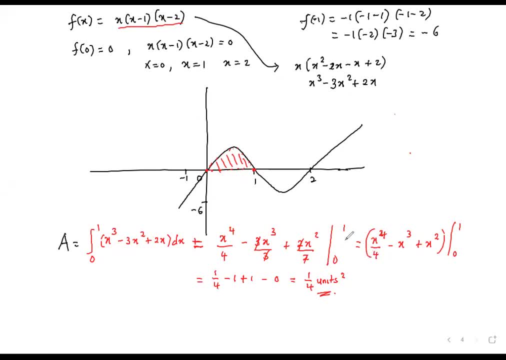 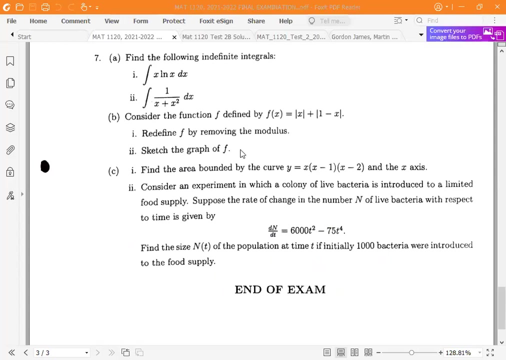 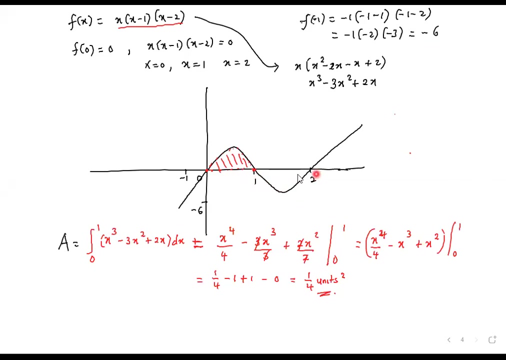 ah, so we need to. let's go back to the question. i think, thank you find the area bounded by this scale and the x-axis. i think we still have a piece that we haven't done, this piece here, this piece here is also bounded by the cave and the x-axis, so it wasn't even ready. 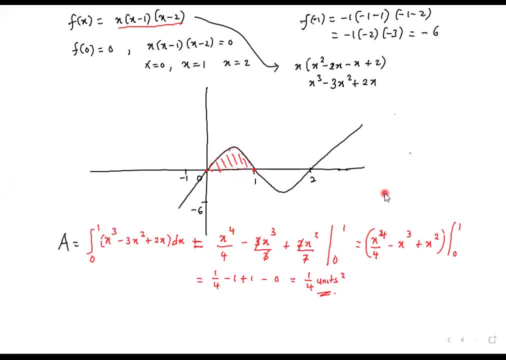 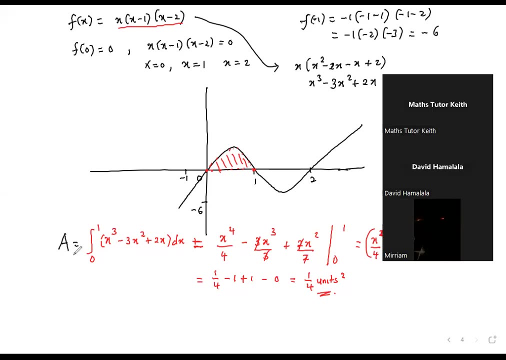 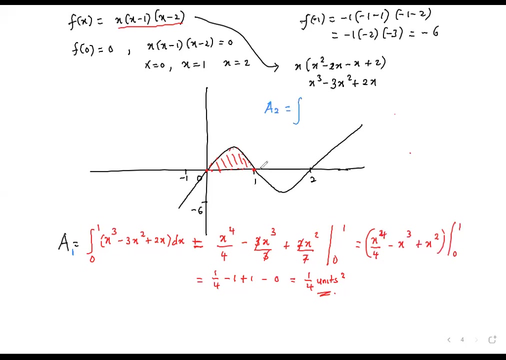 so let's, let's integrate this piece. let me turn the engine so we also integrate this. so say area one then and area two. so area two will be the integral from the curve, which is zero, minus the down care, which is x power 3 minus 3x, squared plus 2x.